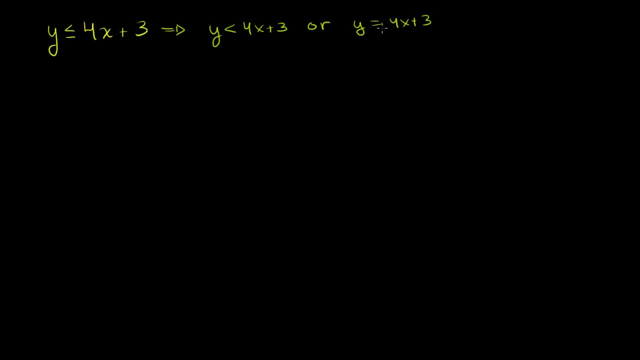 That's what less than or equal means. It could be less than or equal, And the reason why I did that on this first example problem is because we know how to graph that, So let's graph that. So if we try to draw it a little bit neater than that, 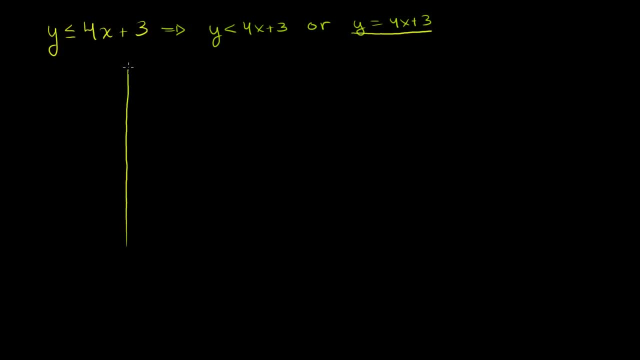 So that is 9.. No, that's not good. So that is my vertical axis, my y-axis, This is my x-axis, right there, That is the x-axis, And then we know the y-intercept. The y-intercept is 3.. 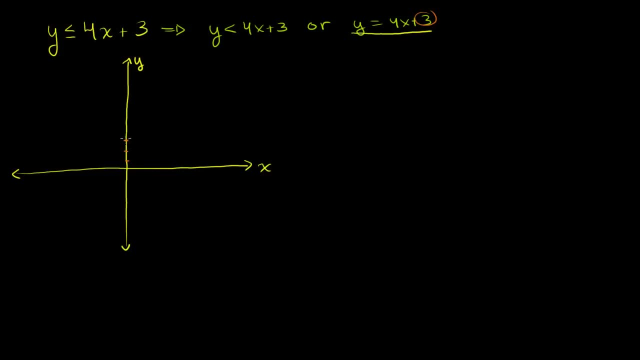 So the point 0,, 3,, 1,, 2,, 3 is on the line And we know we have a slope of 4, which means if we go 1 in the x-direction, we're going to go up 4.. 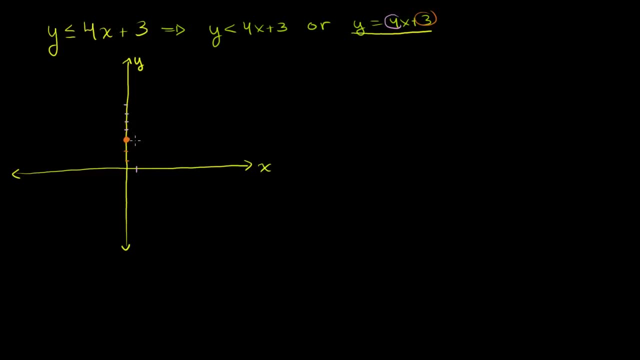 And the y, So 1,, 2,, 3,, 4.. So it's going to be right here And that's enough to draw a line. But we could even go back in the x-direction. If we go 1 back in the x-direction, we're going to. 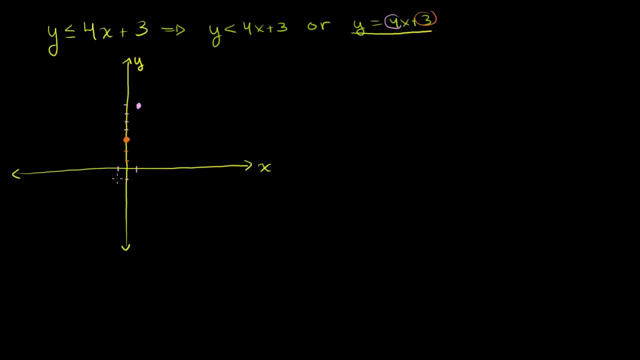 go down 4.. 1,, 2,, 3,, 4.. So that's also going to be a point on the line. So my best attempt at drawing this line is going to look something like something. This is the hardest part. 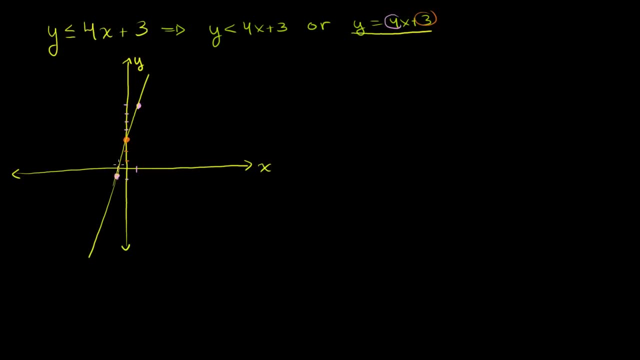 It's going to look something like that. That's the hardest part. That is a line. It should be straight. I think you get the idea That right there is. the graph of y is equal to 4x plus 3.. So let's think about what it means to be less than. 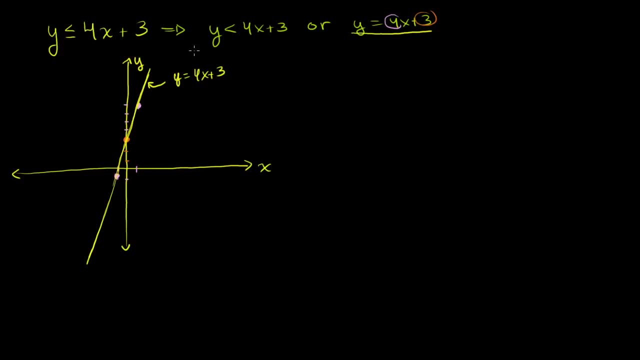 So all of these points satisfy this inequality, But we have more. This is just these points over here. What about all of these where y is less than 4x plus 3?? So let's think about what this means. Let's pick up some values for x. 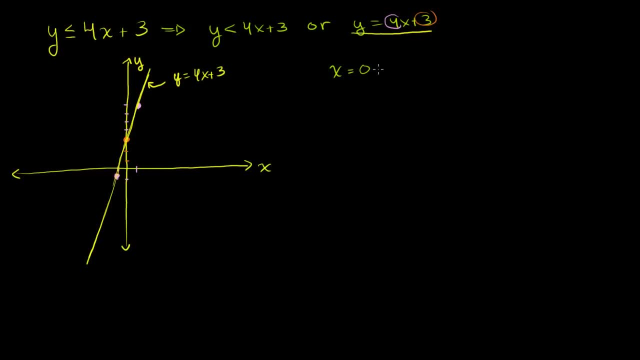 When x is equal to 0, what does this say? When x is equal to 0,, then that means y is going to be less than 0 plus 3.. y is less than 3.. When x is equal to negative 1, what is this telling us? 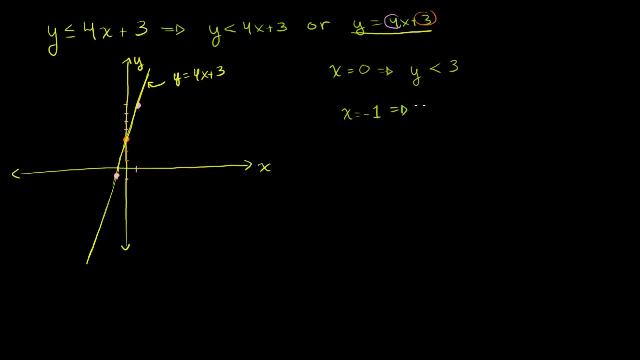 4 times negative. 1 is negative. 4 plus 3 is negative 1. y would be less than negative 1.. When x is equal to 1, what is this telling us? 4 times 1 is 4 plus 3 is 7.. 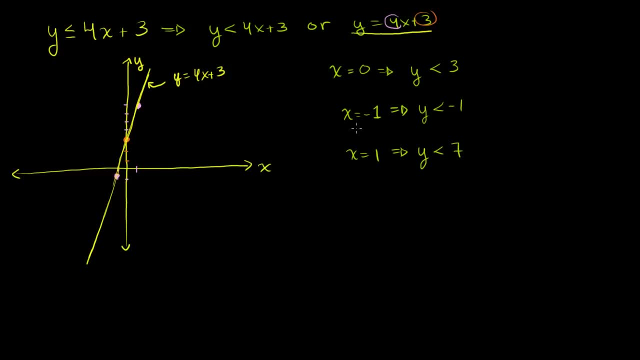 So y is going to be less than 1.. y is going to be less than 7.. So let's at least try to plot these. So, when x is equal to, let's plot this one first. When x is equal to 0,, y is less than 3.. 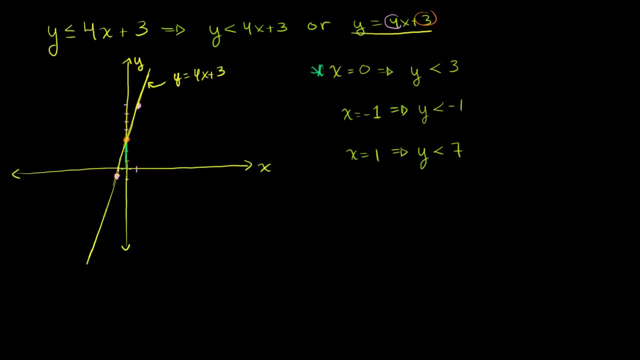 So when x is equal to 0,. y is less than 3.. So it's all of these points here that I'm shading in in green. satisfy that right there. If I were to look at this one over here, when x is negative, 1,. 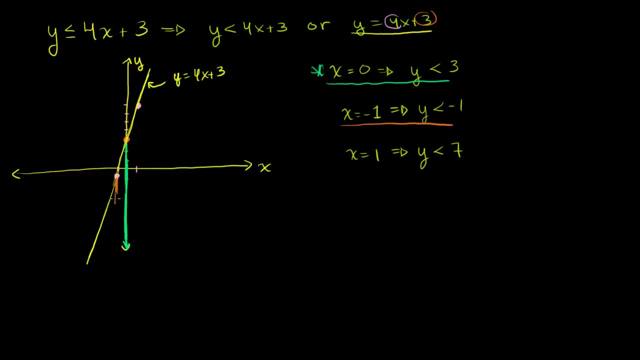 y is less than negative 1.. So y has to be all of these points down here. When x is equal to 1, y is less than 7.. When x is equal to 1, y is less than 7.. So it's all of these points down here. 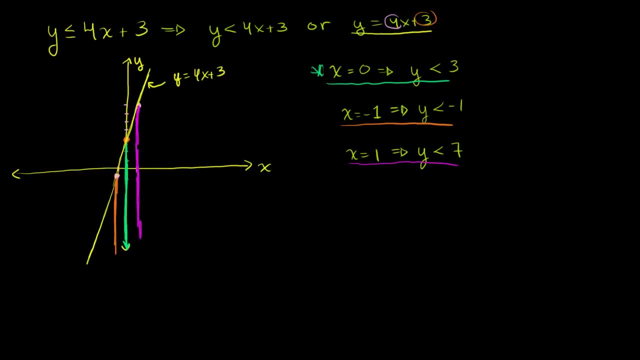 And in general you take any point. you take any point x. Let's say, you take this point x right there. If you evaluate 4x plus 3, you're going to get the point on the line, That is, that x times 4 plus 3.. 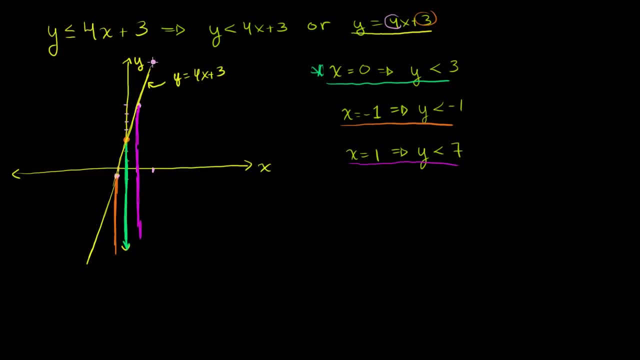 Now the y's that satisfy it. it could be equal to that point on the line, or it could be less than So it's going to go below the line. So if you were to do this for all the possible x's, 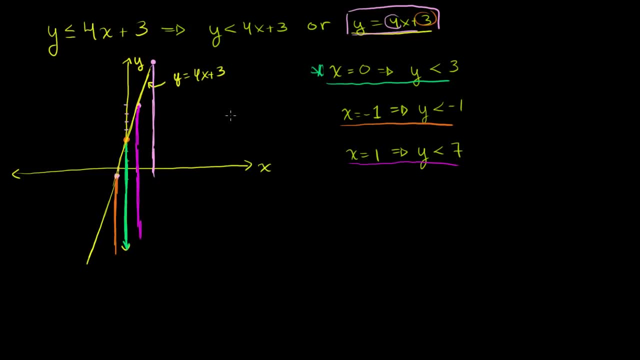 you would not only get all the points on this line which we've drawn, you would get all the points below the line. So now we have graphed this inequality. It's essentially this line- 4x plus 3, with all of the area below it shaded. 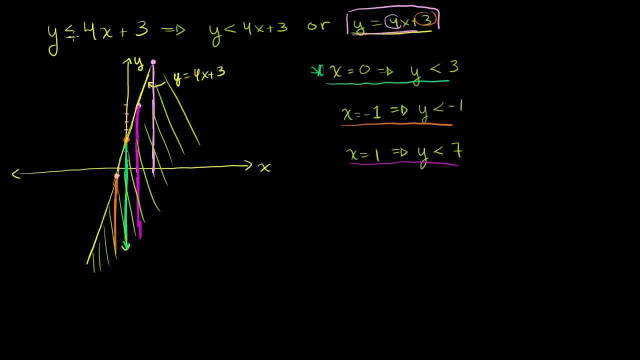 Now, if this was just a less than, not less than or equal sign, we would not include the actual line And the convention to do that is to actually make the line a dashed line. This is the situation if we were dealing with just less. 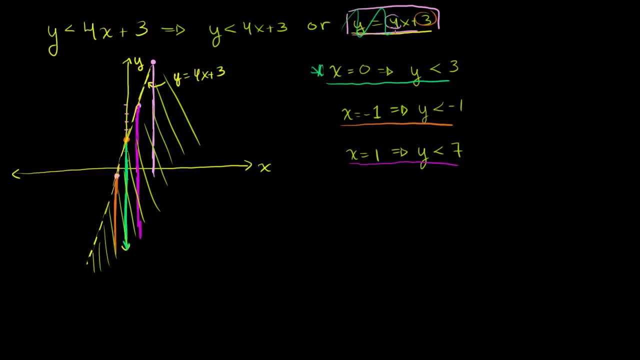 than 4x plus 3.. Because in that situation this wouldn't apply and we would just have that. So the line itself wouldn't have satisfied it, just the area below it. Let's do one like that. So let's say we have: y is greater than negative, x over 2. 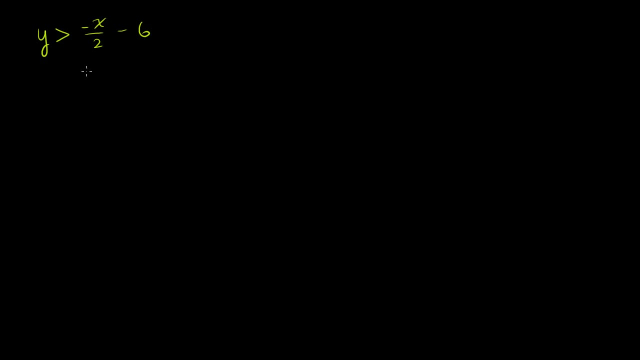 minus 6.. So a good way to start, the way I like to start these problems, is to just graph this equation right here. So let me just graph, just for fun. let me graph. y is equal to this is the same thing as negative 1, half minus 6.. 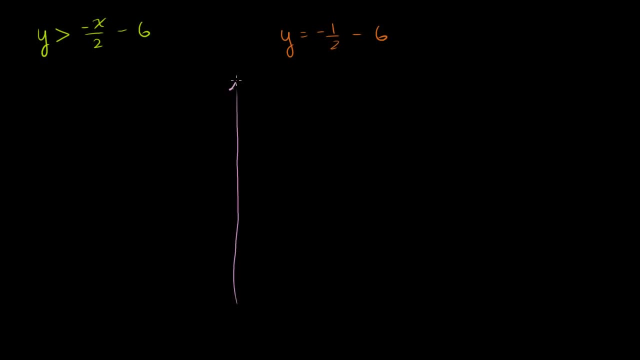 Let me graph it. That is my vertical axis, That is my horizontal axis, And our y-intercept is negative 6.. So 1,, 2,, 3,, 4,, 5,, 6.. So that's my y-intercept. 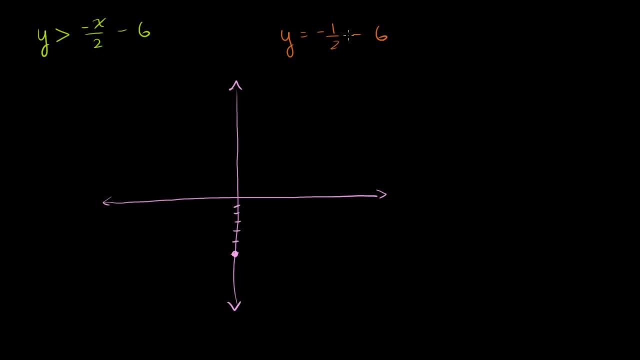 And my slope is negative 1 half. Well, that should be an x there. Negative 1 half, x. Negative 1 half, x minus 6.. So my slope is negative 1 half, which means when I go 2 to the 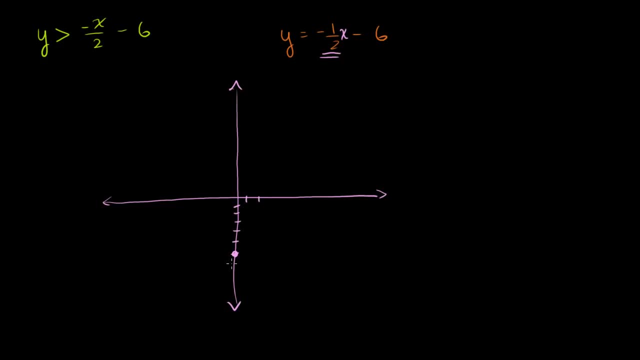 right, Right, I go down Right, Right Down 1.. So if I go 2 to the right, I'm going to go down 1.. So 2 to the right down, 1.. If I go 2 to the left, if I go negative 2, I'm going to go up. 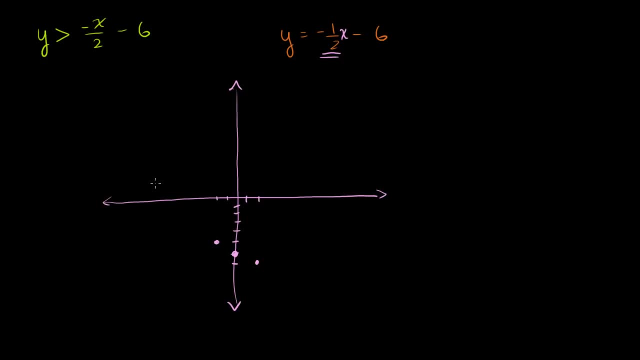 1.. So negative 2, up 1.. So my line is going to look like this. My line is going to look like that. That's my best attempt at drawing the line. So that's, the line of y is equal to negative 1 half x. 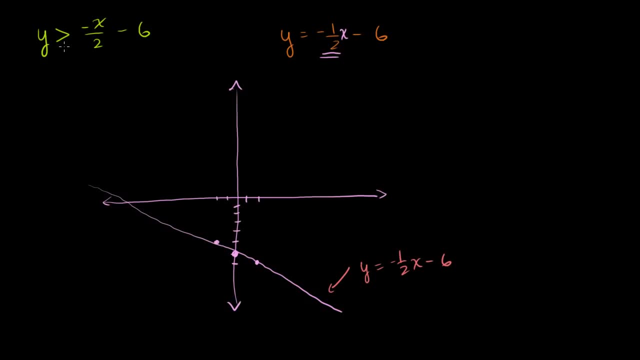 minus 6.. Now our inequality is not greater than or equal, it's just greater. It's greater than negative x over 2 minus 6, or greater than negative 1 half x minus 6.. So, using the same logic as before for any x. 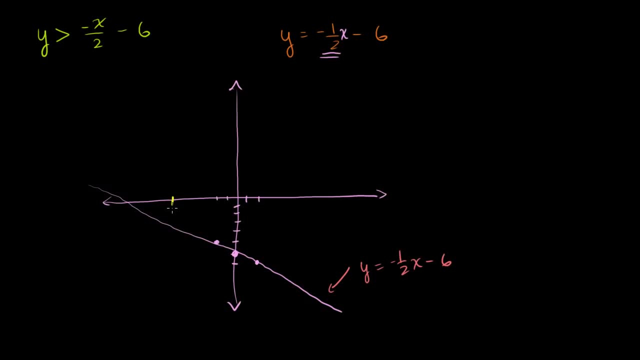 So if you take any x, let's say that's a particular x we want to pick. If you evaluate negative x over 2 minus 6, you're going to get that point right there. You're going to get the point on the line.